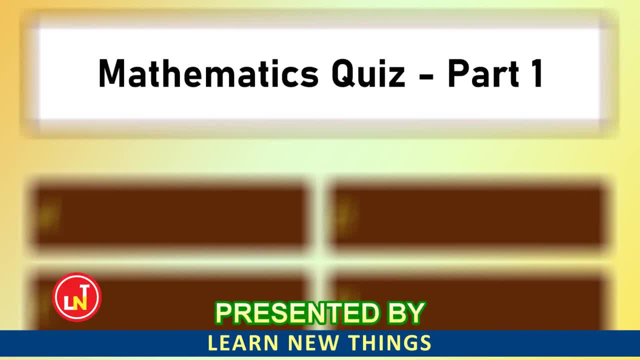 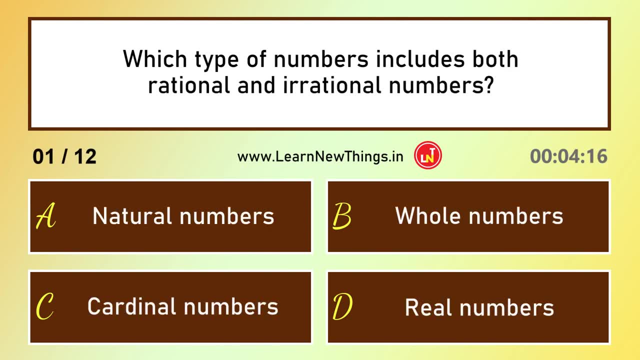 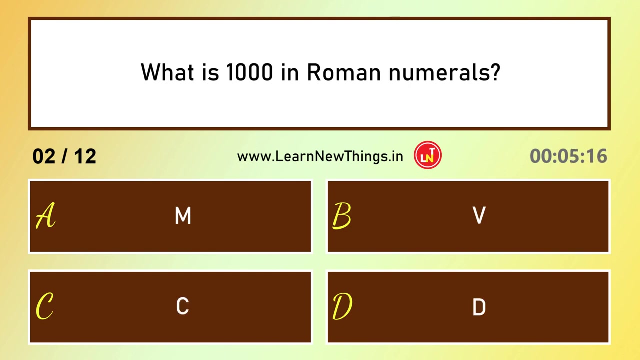 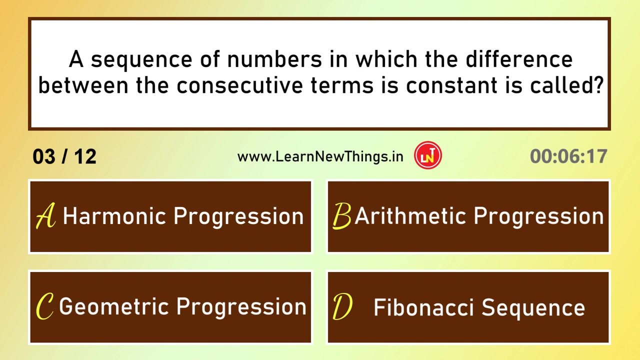 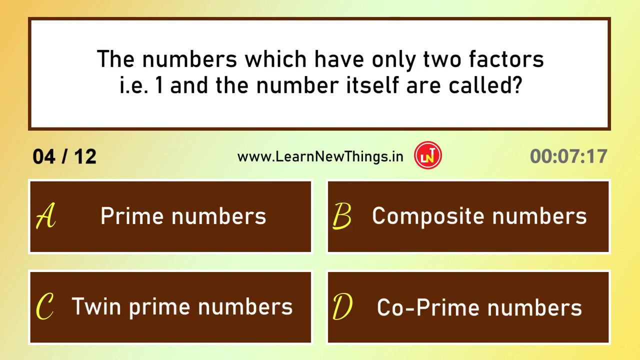 Which type of numbers includes both rational and irrational numbers. Real numbers- What is 1000 in Roman numerals? M? A sequence of numbers in which the difference between the consecutive terms is constant is called arithmetic progression. The numbers which have only two factors, ie 1 and the number itself, are called 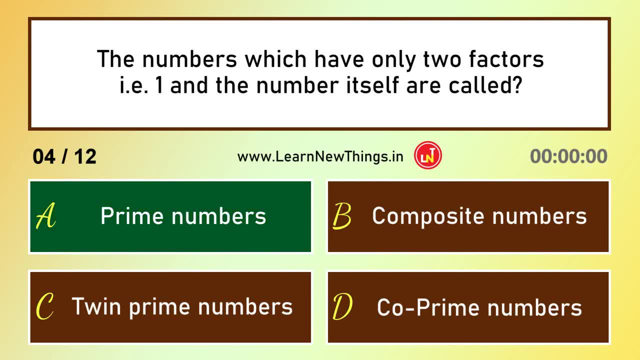 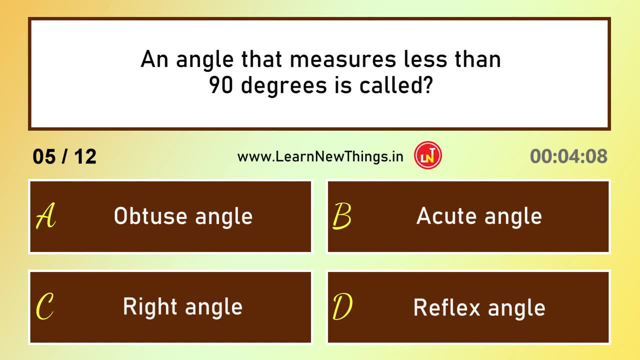 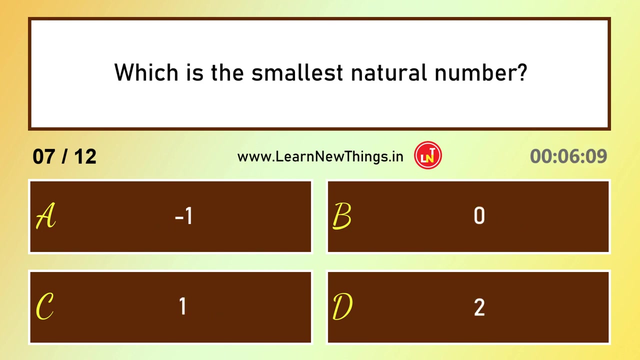 prime numbers. An angle that measures less than 90 degrees is called acute angle. The number that is left after the division process is called remainder, which is the smallest natural number. 1. The straight line segment joining any two points on the circumference of the circle is called 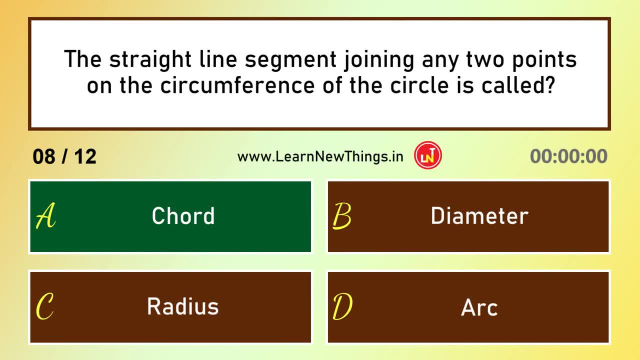 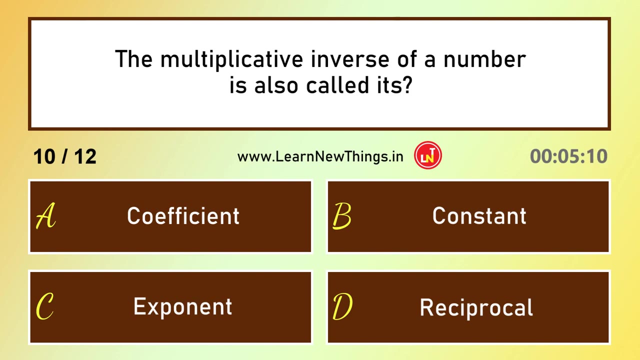 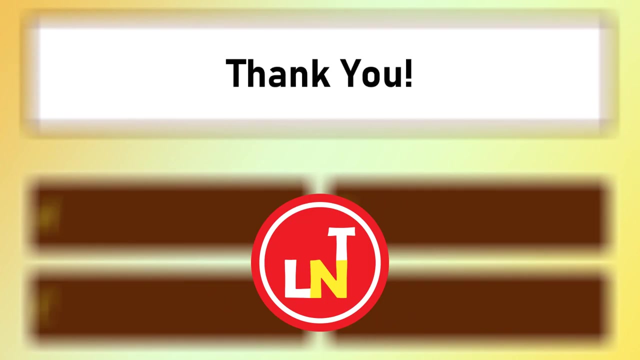 chord, which is the longest chord of a circle Diameter. The multiplicative inverse of a number is also called its reciprocal. What is the reciprocal of 1 by 2?? 2, The square root of the variance, is called standard deviation.